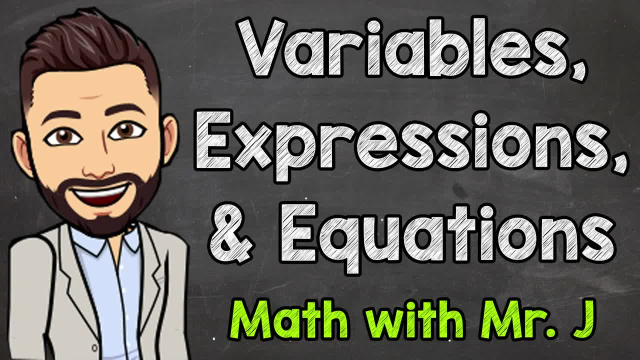 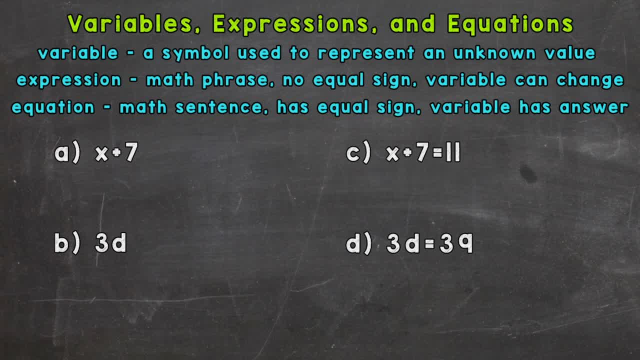 Welcome to Math with Mr J. In this video I'm going to cover variables, expressions and equations. So let's start with variables. And a variable is a symbol used to represent an unknown value, And variables are usually represented by a letter. Think of a variable. 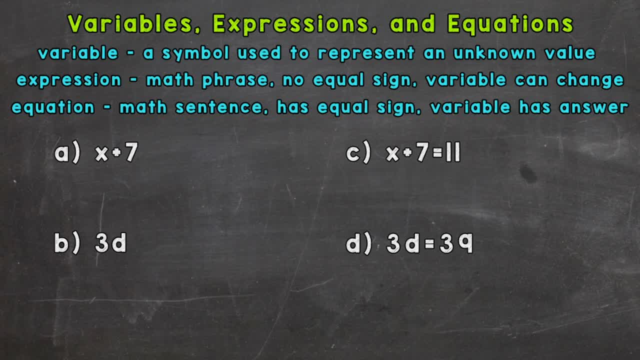 like a missing puzzle piece within a math problem. Now, a variable's value can change or it can be defined, which means a set value depending on the context or situation. We'll talk a little more about that later. Then we have expressions, and an expression is a math phrase. There's no equal sign. 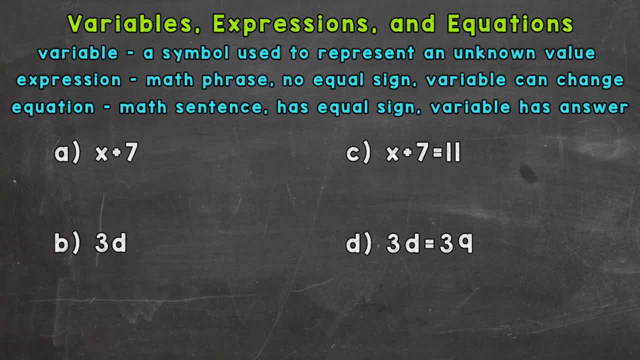 and this is the situation where the variable can change values. And lastly, we have equations, Equations you can think of like a full math sentence. It has an equal sign and variables have a defined or set answer. So when I mentioned that an expression is like a math phrase, think of that like an expression is part of a math sentence and an equation is that full math sentence. 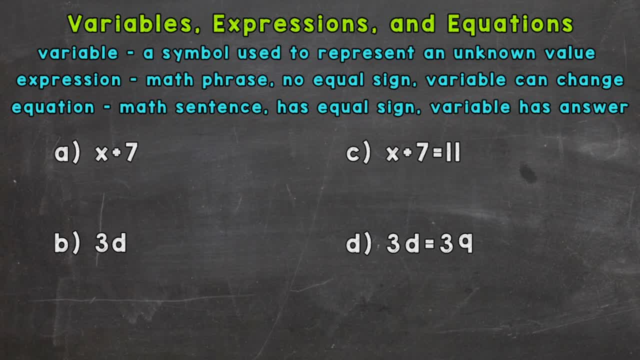 So let's jump into the examples down below. So examples A and B are expressions. It's a math phrase. There's no equal sign and the variable can change. So for example A, here maybe x, is equal to 5.. So if x equals 5 and we plug 5 in for our variable and solve, we would get an answer of 12.. 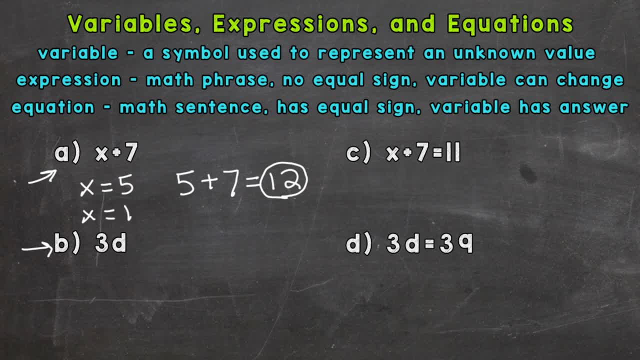 Or maybe x is equal to 13 here. So if x equals 13,, we would have 13 plus 7 and we would get a solution or answer of 20.. Example B: Example B: here we have 3d. So whenever you have a number right next to a variable, right next to a letter, it means multiplication. 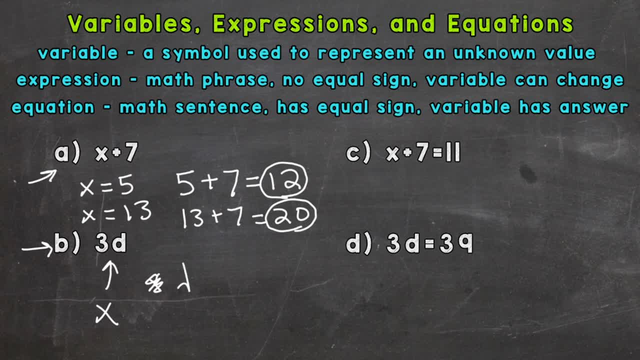 So if x or, I'm sorry, if d equals 11,, we would plug that in 3 times 11, and we would get 33.. So again, A and B are expressions, Now C and D are equations. And how you can remember this? equations have equal signs. 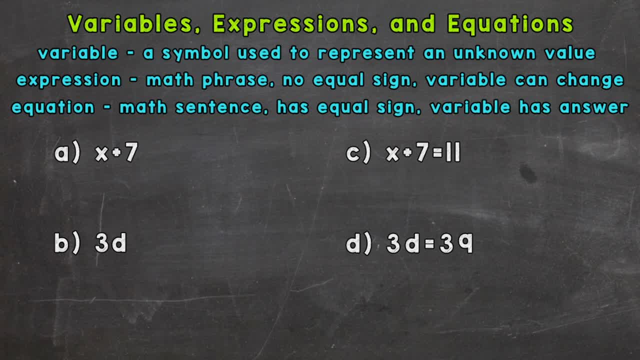 and this is the situation where the variable can change values. And lastly, we have equations, Equations you can think of like a full math sentence. It has an equal sign And variables have a defined or set answer. So when I mentioned that an expression is like a math phrase, think of that like an expression is part of a math sentence and an equation is that full math sentence. 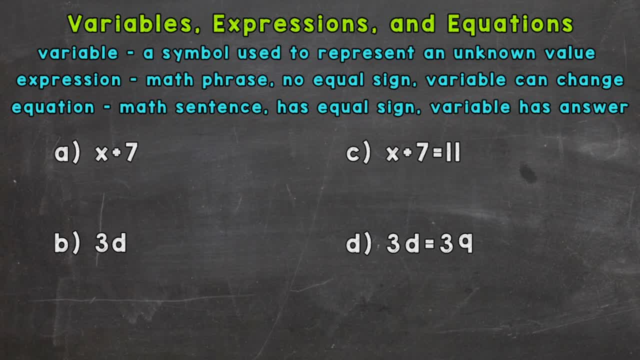 So let's jump into the examples down below. So examples A and B are expressions. It's a math phrase. There's no equal sign and the variable can change. So for example A, here maybe x, is equal to 5.. So if x equals 5 and we plug 5 in for our variable and solve, we would get an answer of 12.. 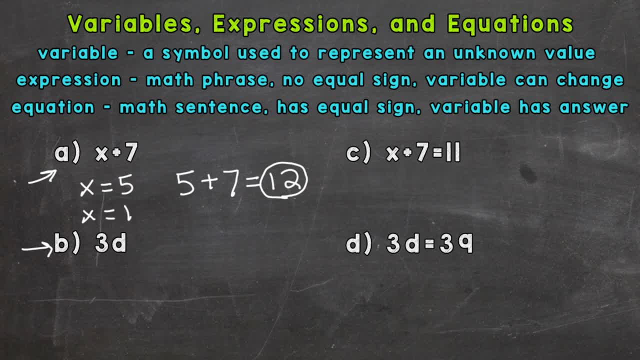 Or maybe x is equal to 13 here. So if x equals 13,, we would have 13 plus 7 and we would get a solution or answer of 20.. Example B: Example B: here we have 3d. So whenever you have a number right next to a variable, right next to a letter, it means multiplication. 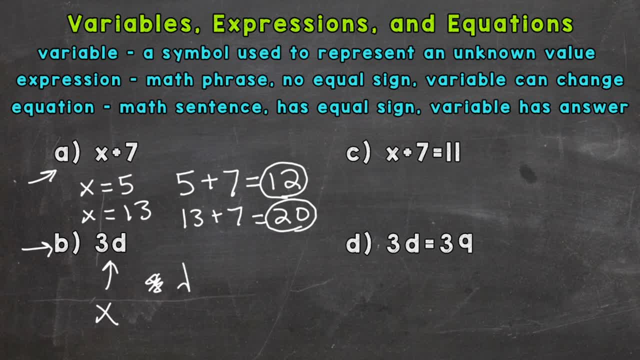 So if x or, I'm sorry, if d equals 11,, we would plug that in 3 times 11, and we would get 33.. So again, A and B are expressions, Now C and D are equations. And how you can remember this? equations have equal signs. 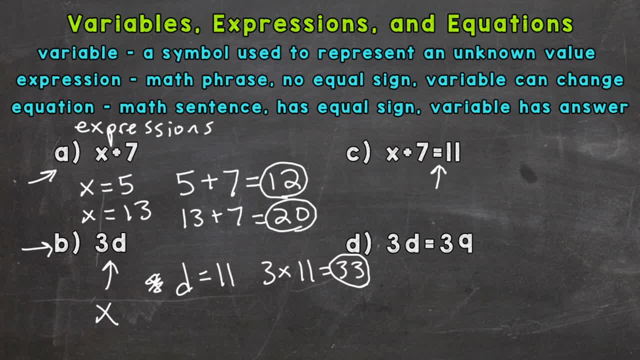 So equations have equal signs, expressions don't, So these: the variable has a defined or set value. We can't say x equals 5 here, like we did for letter A, example A, Because if we plug 5 in we do not get 11.. 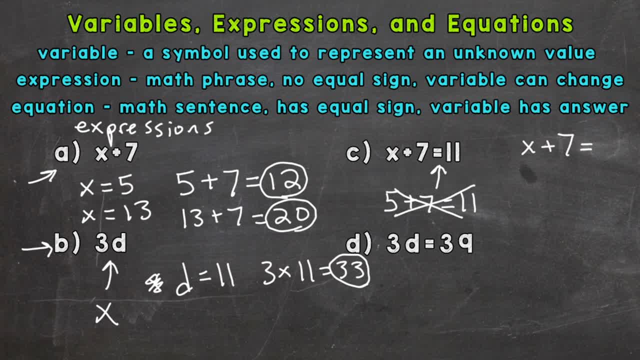 We would have to solve For this variable- or you can probably do this- one mental math. So we need to isolate the variable, subtract 7 from both sides and we get x equals 4.. x can only equal 4 here.